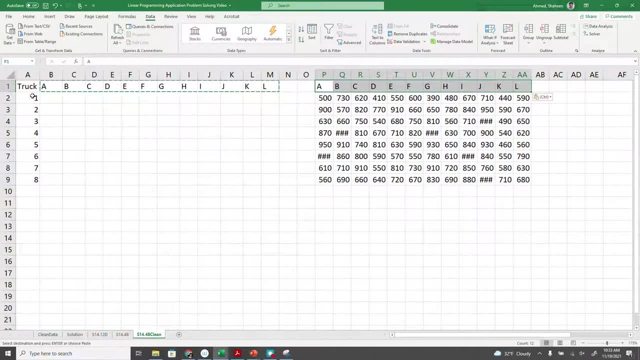 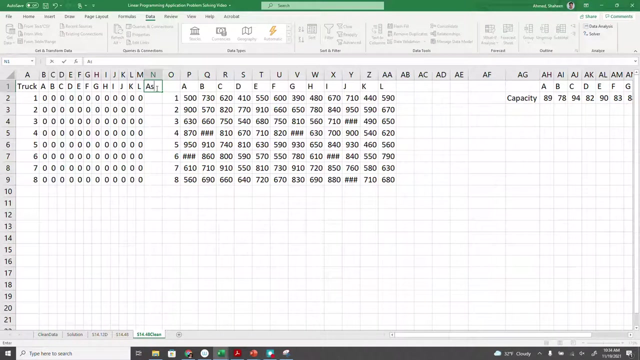 there So I know whose mileage is what, and also copy this track right here. so this, the server function in excel, will start with zeros and then it will fill with some number after performing all the operations behind the scene. so i'm going to name this cell as a sign. um, i think, gn, whatever, doesn't matter. 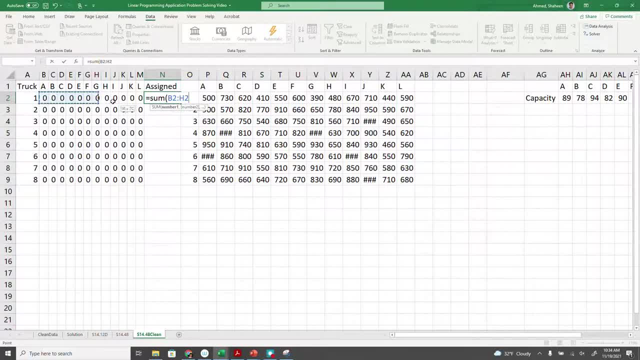 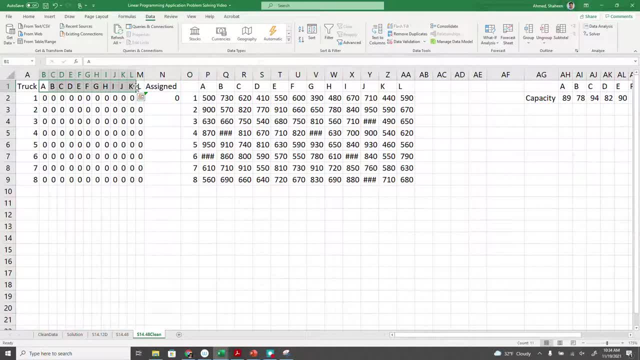 to be more than one. so they're going to be more than one. so they're going to assign this track number one to one of these customers. so in the constraint in the solver we'll put that this sum is exactly equal to one and copy down, and then, similarly, this will be less than or equal to one, because not all. 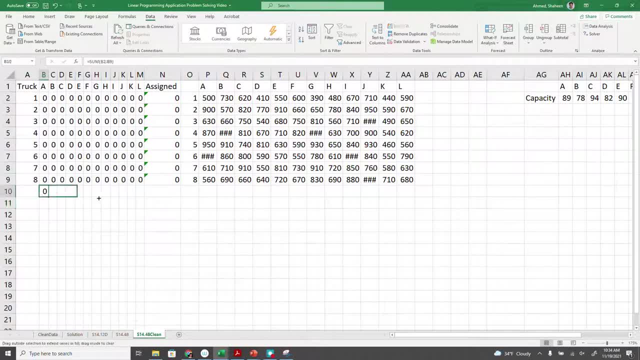 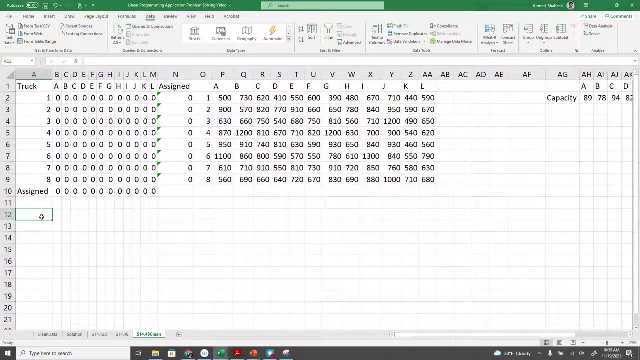 the customer will receive trucks, because we only have eight trucks to assign. also, again, we'll say: assign here and then, um, we'll calculate the total mileage here. so, simply is equal to some product, um, all of these. so there will be only eight ons here and everything else will still be zeros. 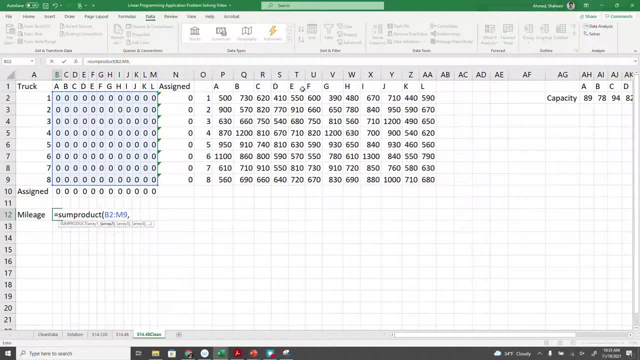 uh, because we have only eight tracks and whatever that track we assign to a particular customer, it will multiply that mileage corresponding mileage and give us the total miles. so we have total eight um trucks mileage there and now they have a capacity constraint that they don't want to send to the track to a customer who does not provide a whole. 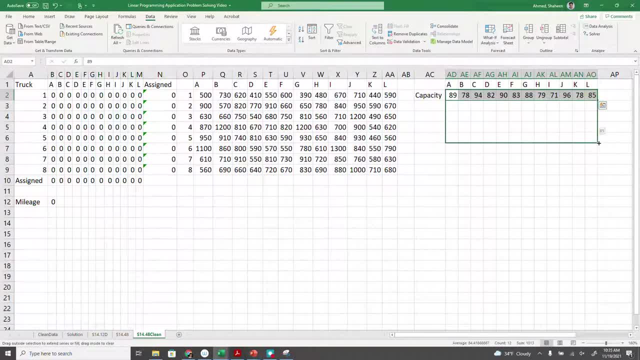 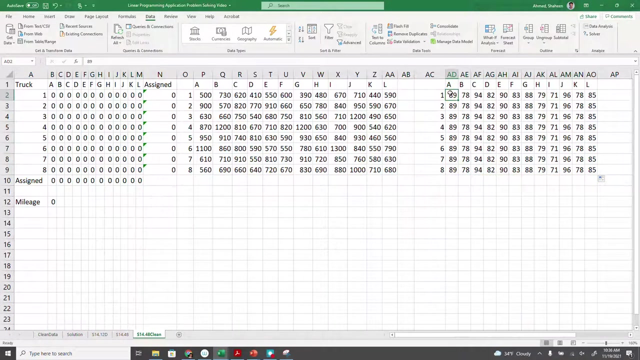 lot of uh goods. so they understand the person, the customer going to make more. so i'm going to do one, two. so this is the capacity given for um these customers. so, for example, customer a, if you send a track to that customer, they will only feel 89 of the truck and about 11 will be empty. 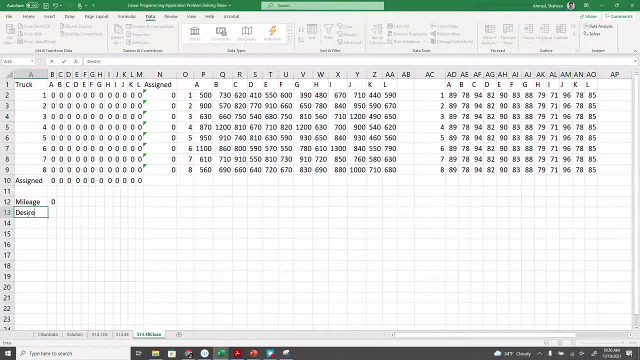 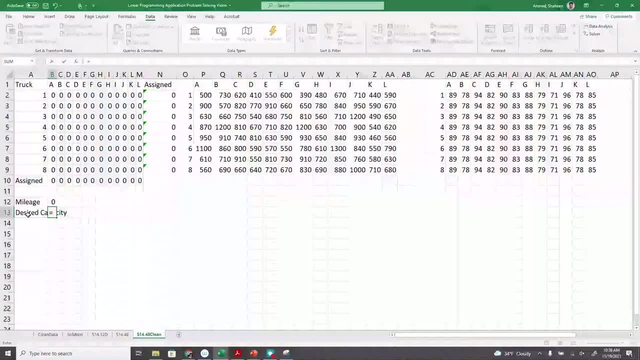 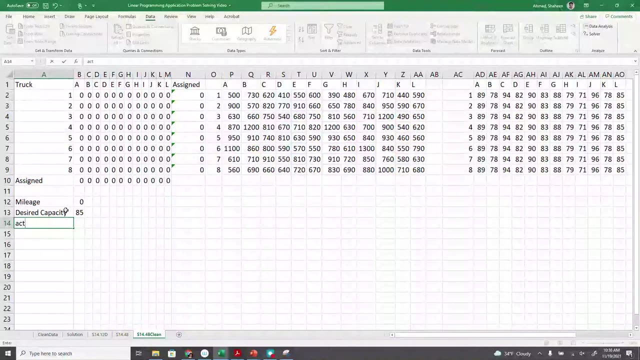 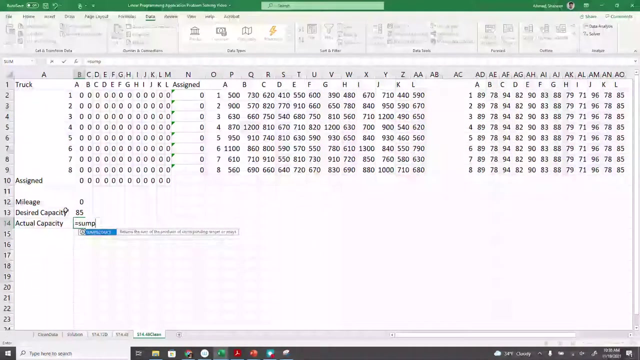 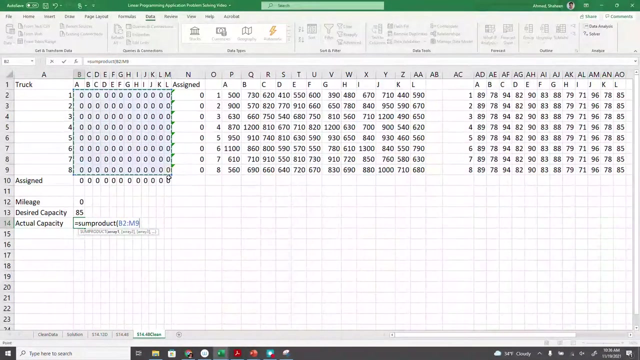 and their desired capacity. so they want to have at least 85. that's given in the problem. you can go back to there and then actual, we're going to calculate using that some product function. we'll simply do some product of this. so whatever track we assign to which customer. 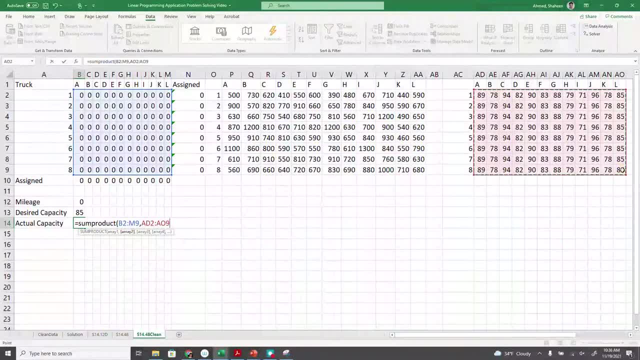 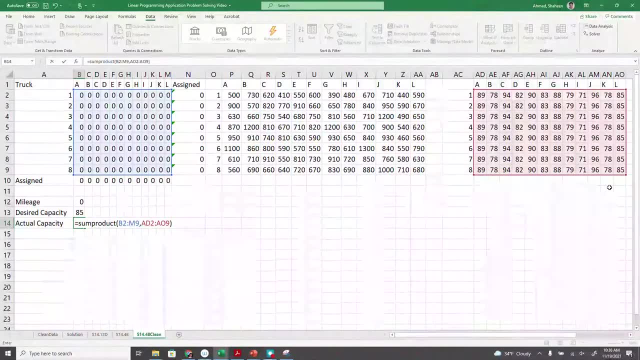 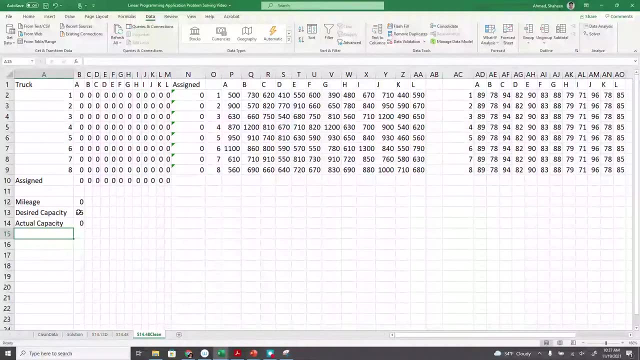 it will multiply with the corresponding number here to find the actual and capacity. now these are eight numbers. so because we have eight tracks, we'll divide by eight to have an average capacity, because this 85 is the average capacity given um for the desired they want to achieve at. 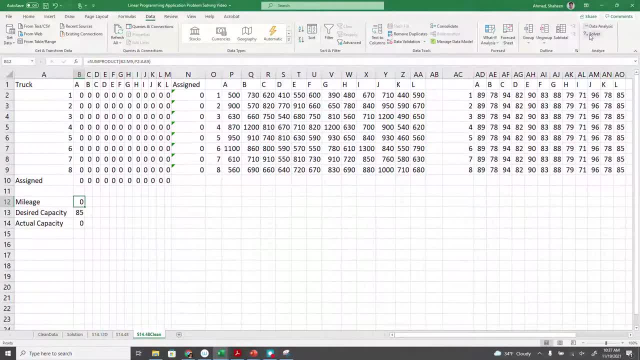 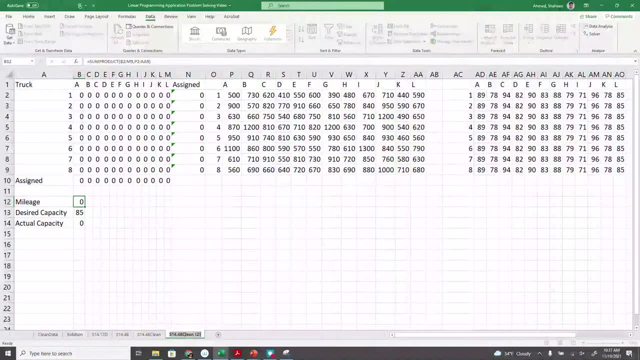 least that capacity. so we have all these things set. now we can go to the solver function. before we go that, i would like to make a copy of this file so in case if i mess up, i can come back and work on. i don't lose anything, because after i solve all, this number will be replaced by something. 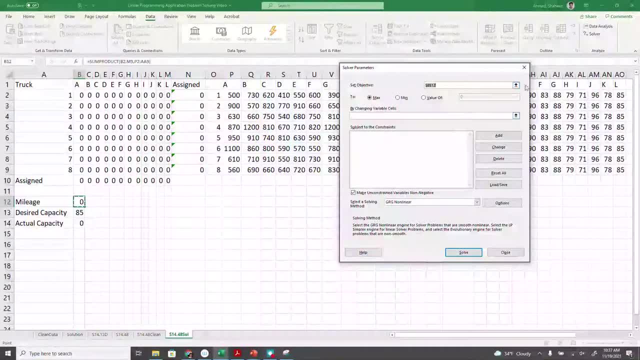 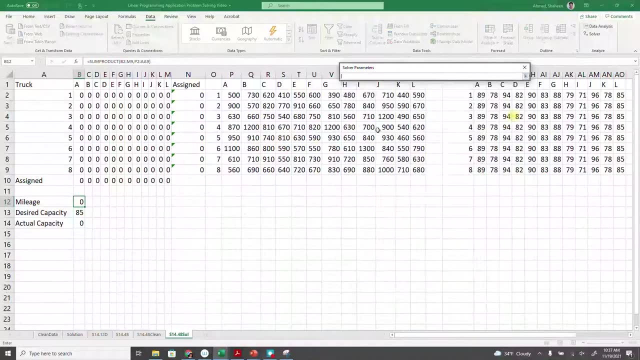 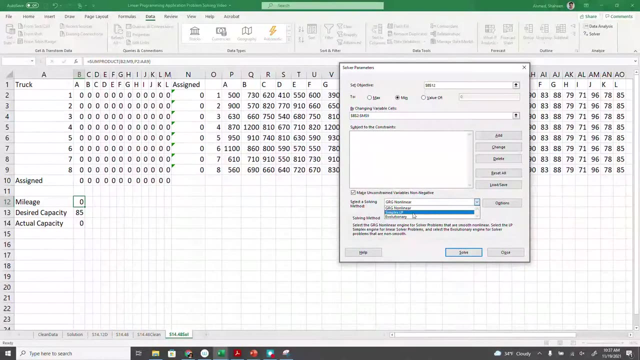 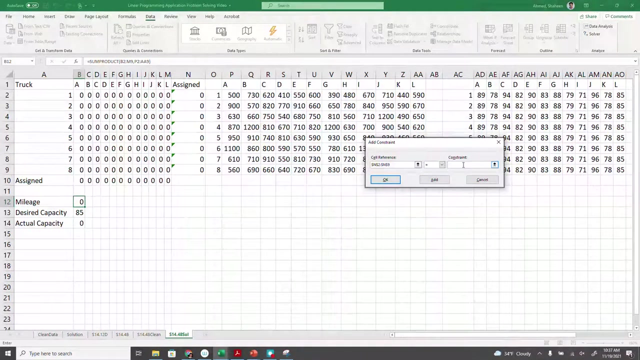 um new. so solver, we're going to minimize. the desired max is select by default. so select the minimize and then it will change these variables. and then i'm going to use the simplex linear programming: add the constraint, so this should be exactly equal to one. we have to add also one more constant for this: that none of these can be a half track. so they're. 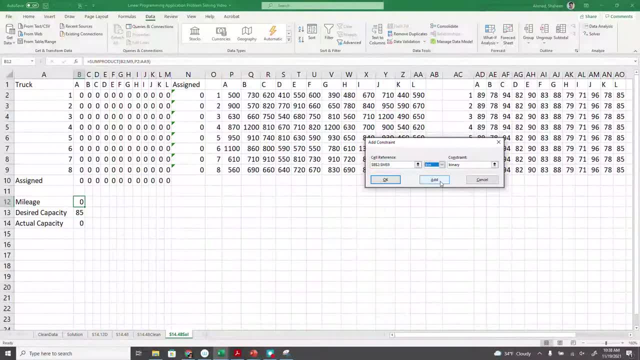 either zero or one, so it's a binary. we want only binary variables there. add, and also: this should be less than or equal to one, because we don't have enough trucks to provide all the customers. and then one more constraint: this should be more than equal to. 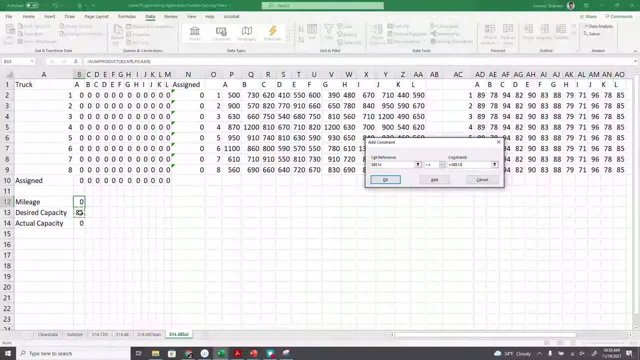 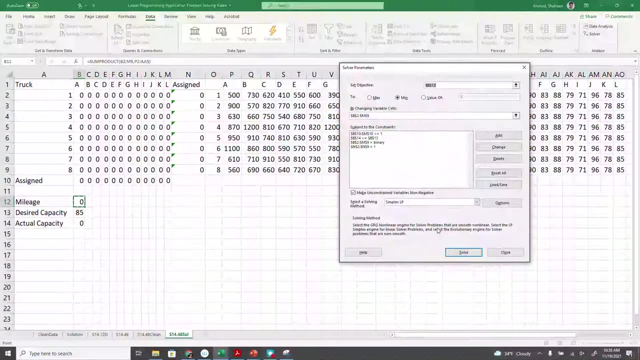 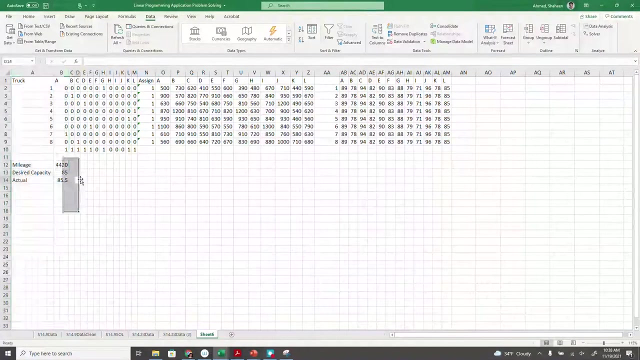 that desired capacity. so we want to achieve at least 80 percent, 85 percent capacity. so i think that's all these. why do i have the? let me do that again, so that, okay, i think that's all. so that's the solution to this problem.